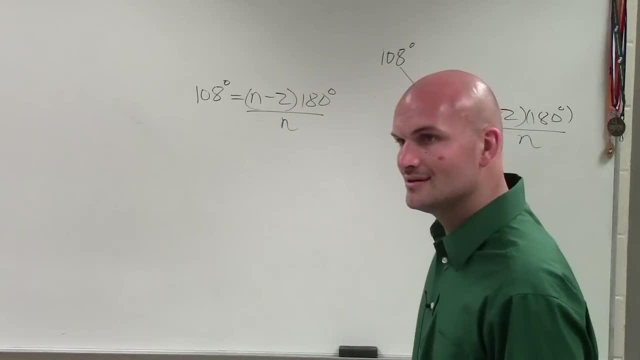 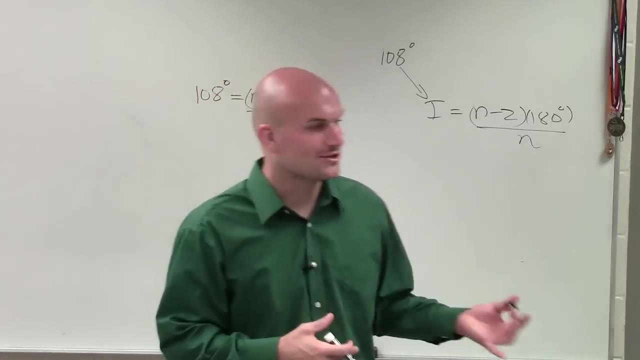 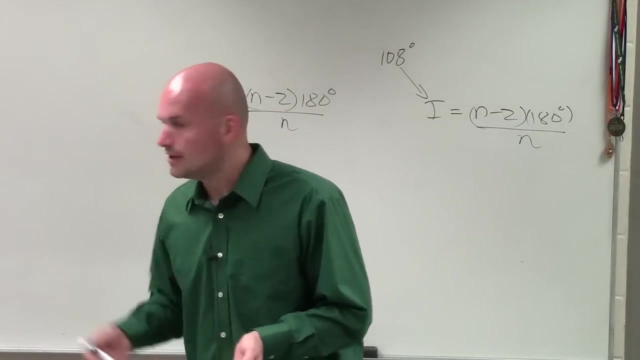 So what represents the number of sides? n? n represents the number of sides, right? So I need to solve for n. Now, guys, going back to your Algebra 1 class, we're solving for a variable. We have to get that variable isolated by itself. 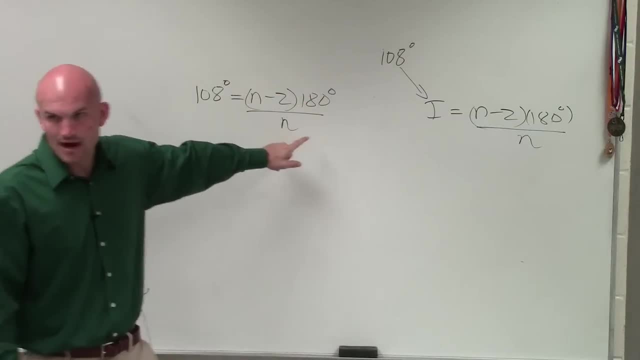 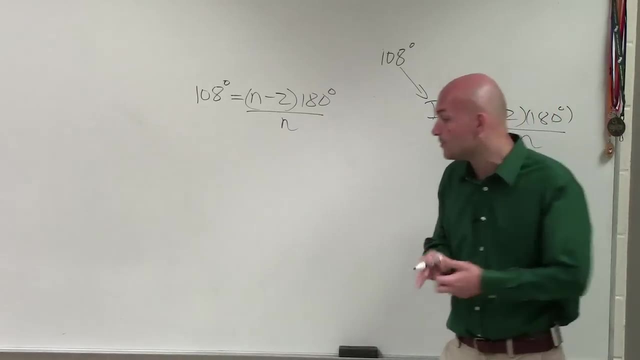 Well, the first thing we need to do is we need to get off the denominator. So how can I get it? How can I get it off of the denominator? What inverse operation can I use? Amber Multiply by n on both sides right. 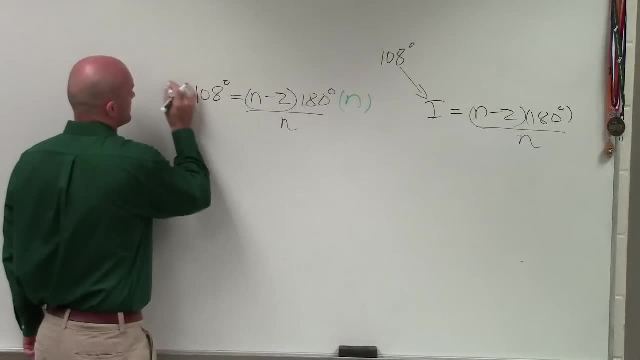 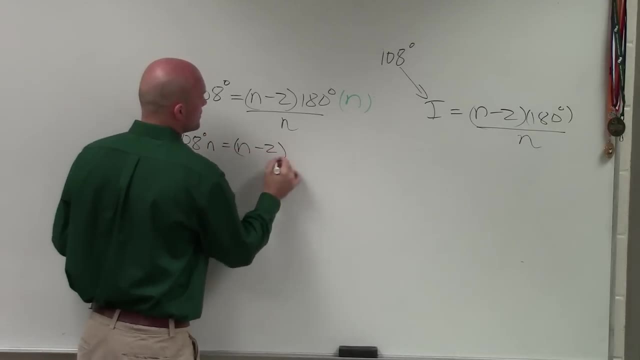 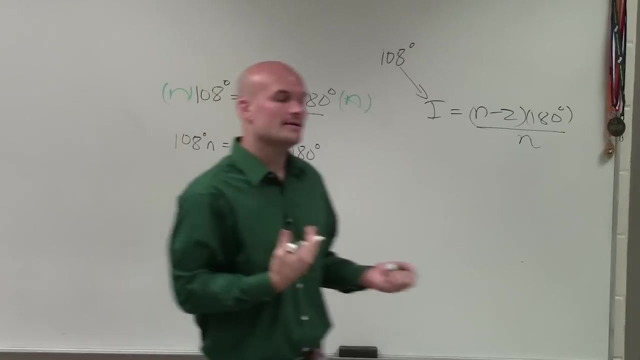 So what I'll do is I'll multiply by n on both sides. Therefore, I have 108n equals n minus 2 times 180 degrees, Because n divided by n just goes into 1.. Now what I can do is I can apply the distributive. 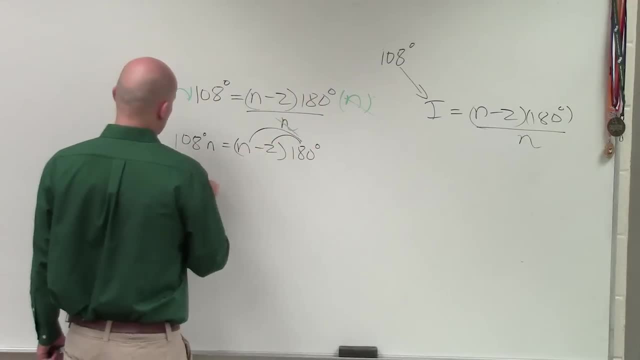 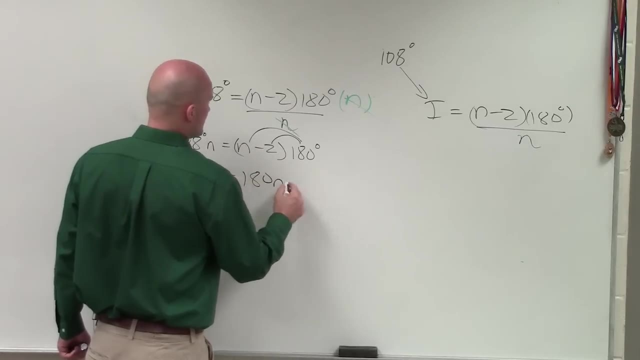 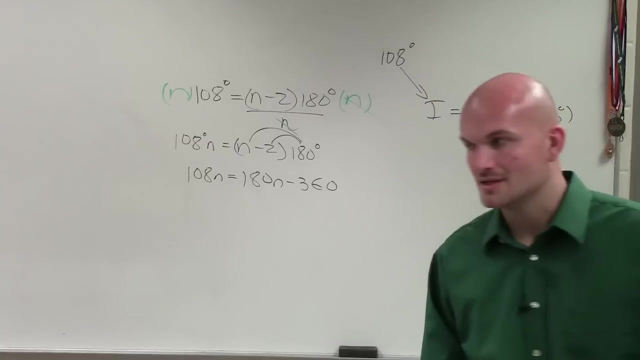 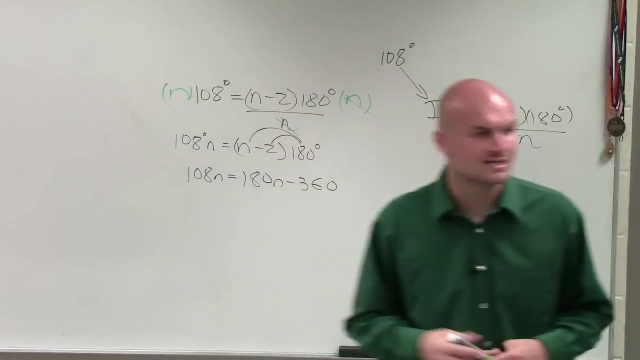 property And therefore I have 108n equals 180n minus 360.. And now we have a variable on both sides. So to get the variable off both sides we have to go and add or subtract to get them on the same side. 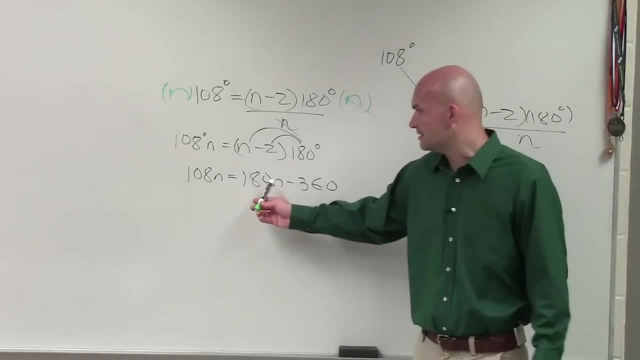 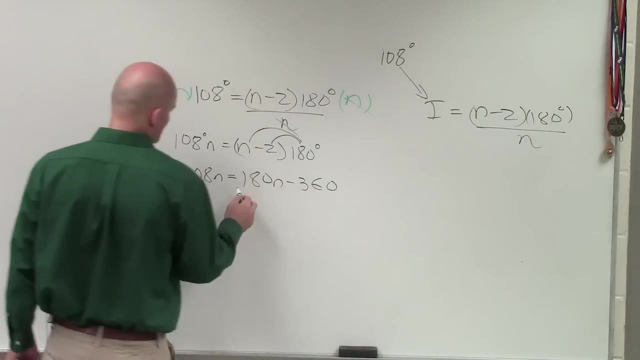 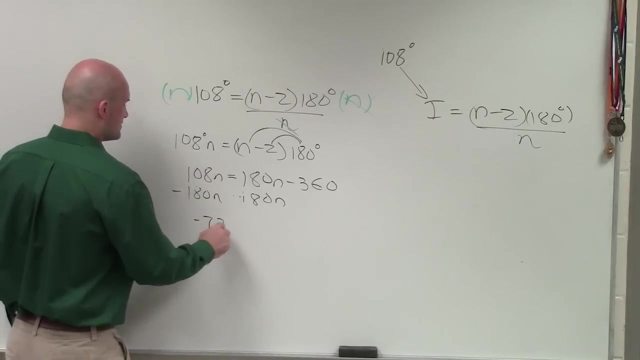 Now, usually what I like to do, ladies and gentlemen, is we can just subtract this over to there, just to get them onto the same side, And that's what I'll do. I'll subtract 180n. Therefore, that's going to give me a negative 72n equals. 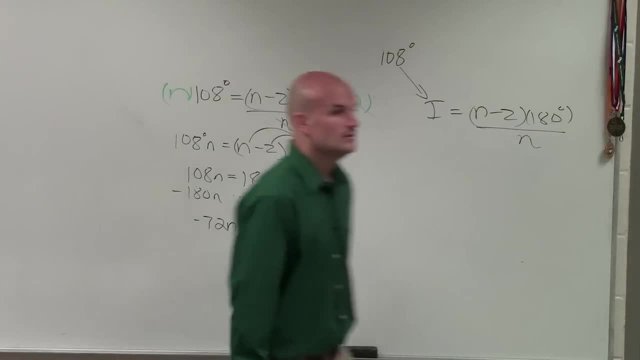 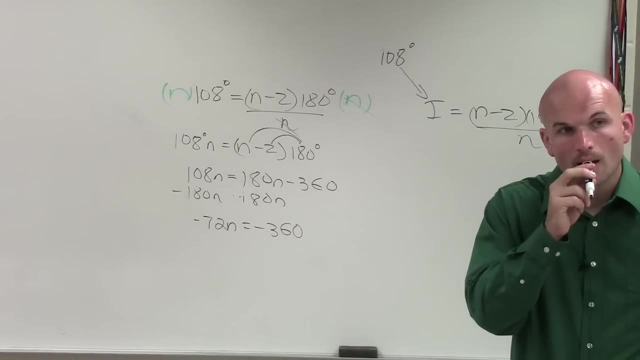 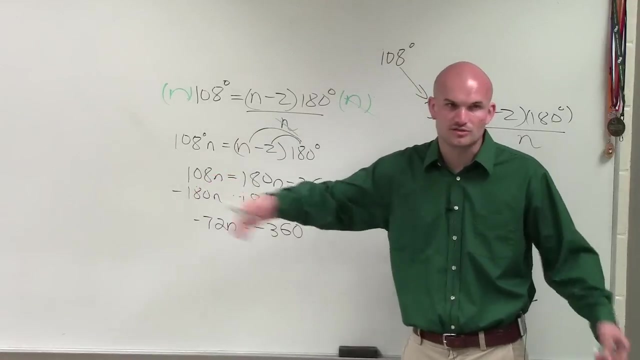 negative 360. Yes, 4.. I know I thought you were supposed to subtract the smaller one. You can. You could subtract the 108 over there and then add 360 to the other side. There's not a problem with that either. 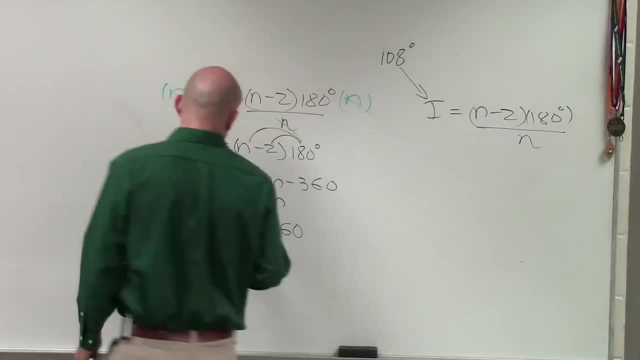 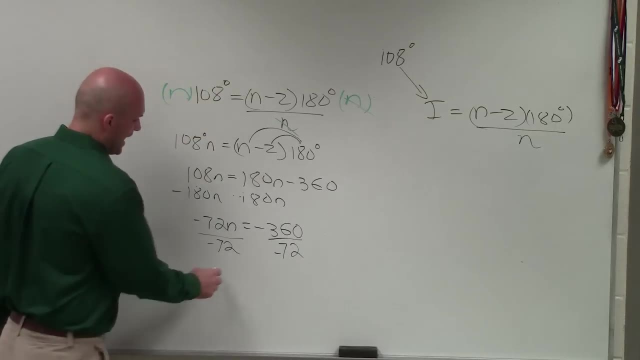 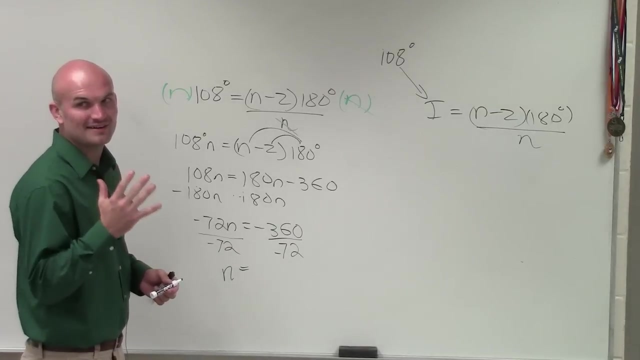 But it doesn't have to be one way or the other, You can really choose. Then I'll just divide by negative 72.. And therefore n equals anybody, Anybody, Anybody, Anybody, 5.. aviator 5?. 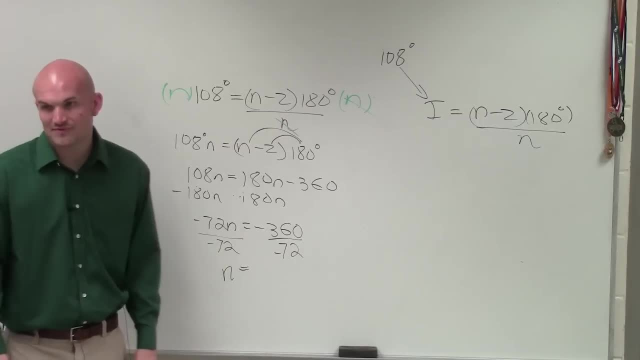 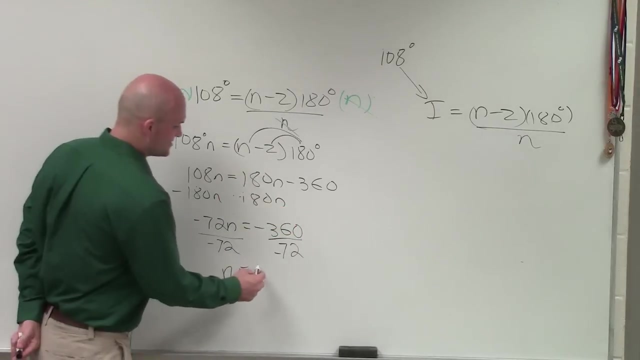 Mystery Student Tetsanikoi. Well, what is seven times 5? 35.. So 5 times 70 would be 350.. Then you have a 2.. 5 times 2 is 10. 360.. So n equals 5.. 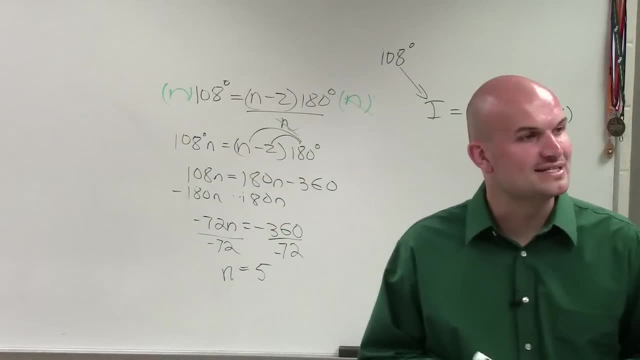 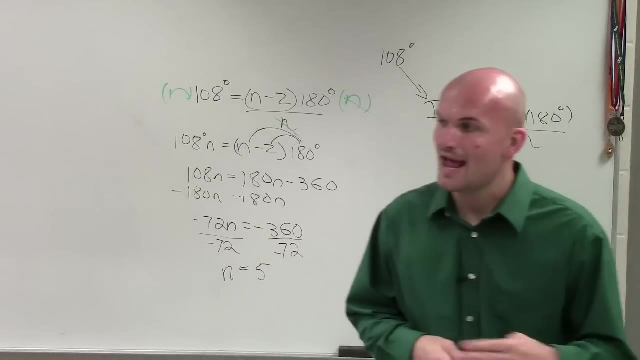 Therefore, if every individual angle is equal to 108 degrees, if each individual angle is equal to 108 degrees, Please他们 personas que son 5. and 8 degrees. you then have a what do we name a five-sided figure. 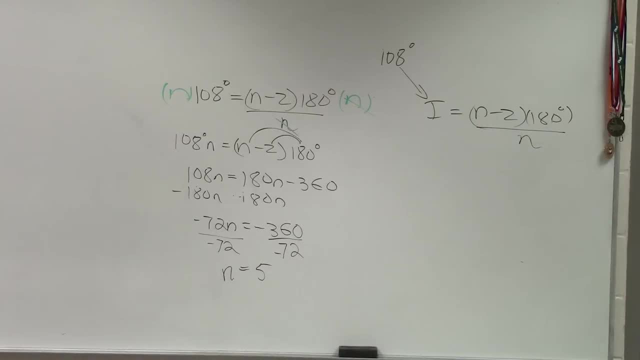 Pentagon Very good. No, it's positive Because a negative? 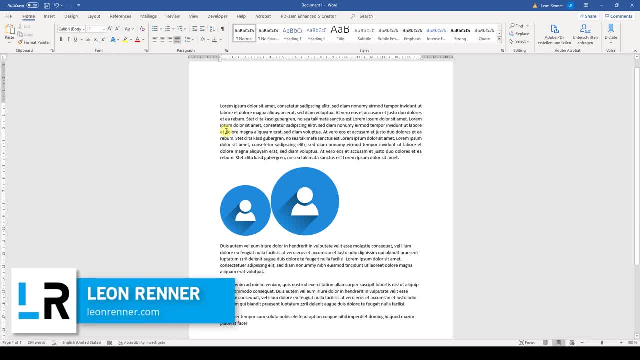 How to group multiple pictures in Microsoft Word. To group the pictures we first have to change the layout options of the pictures. So we click on the picture and then this layout options button will appear in the top right corner. If you don't have this button, go to the picture tools and there 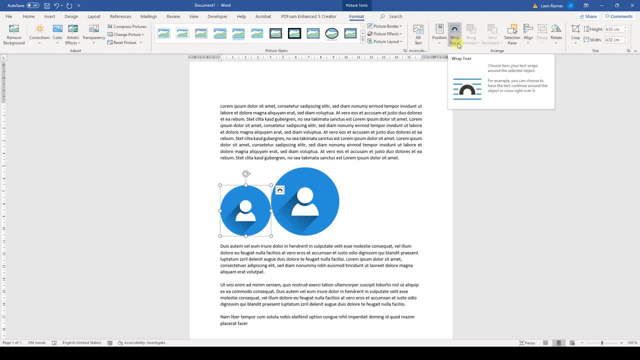 to the format tab and here you will have the same button, but it will be called wrap text. Now we simply click on this button and here we have to choose one of these text wrapping options, So not the original option, but one of these text wrapping options. 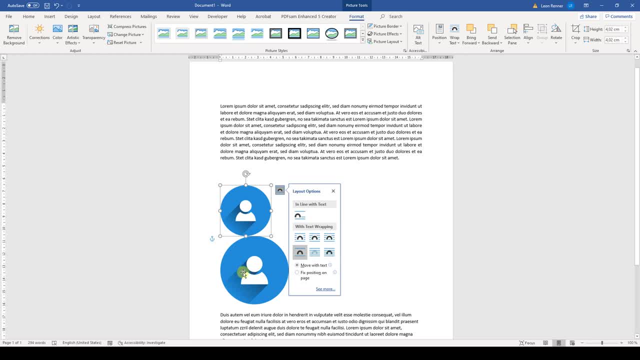 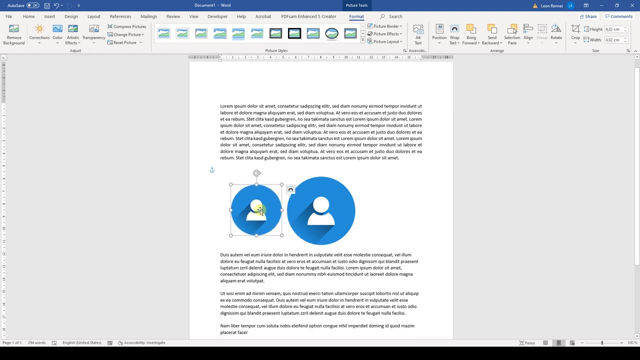 I will choose top and bottom in this example, and then we also have to do the same for the next image. So I will also change the layout options here And now we can position this image freely and also the other one, and to now group them, we select one of the images. 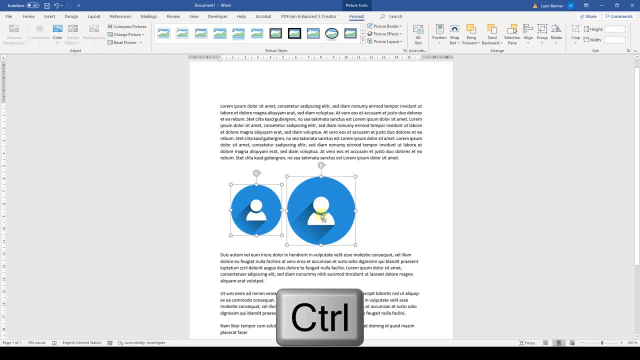 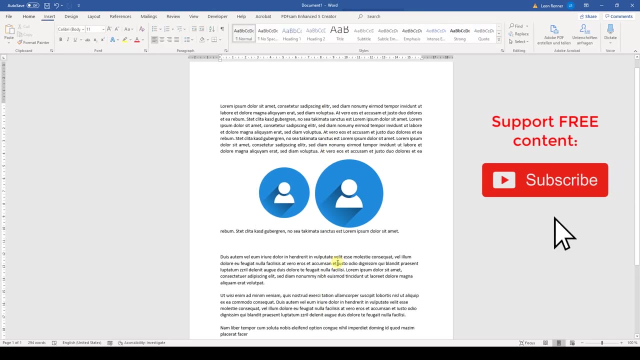 hold down the control key, then select the other image, And when we now do a right-click one of these images, we can select, group and then group again, and these images will be grouped together and here we can now move them as one unit. and that's it. now you know how to group.